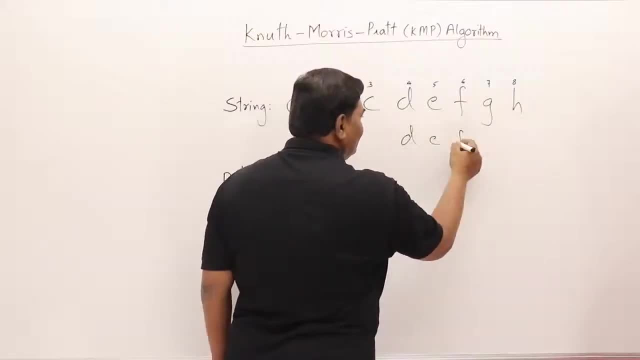 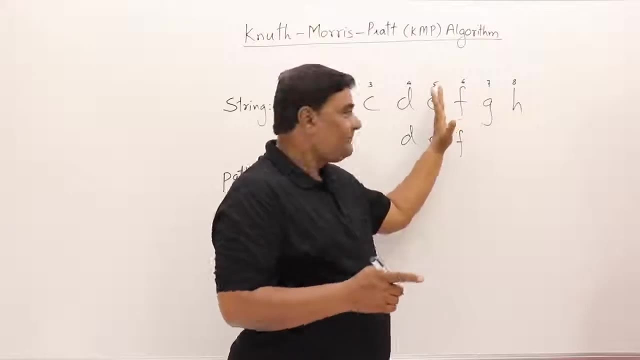 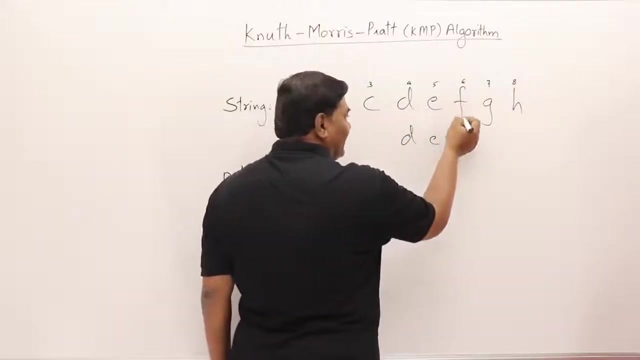 so shift the pattern by one step. This is matching, No need to shift. Check the next, That is also matching. And check the next- This is also matching. So, yes, a pattern is found inside the string, at this place, at this index, that. 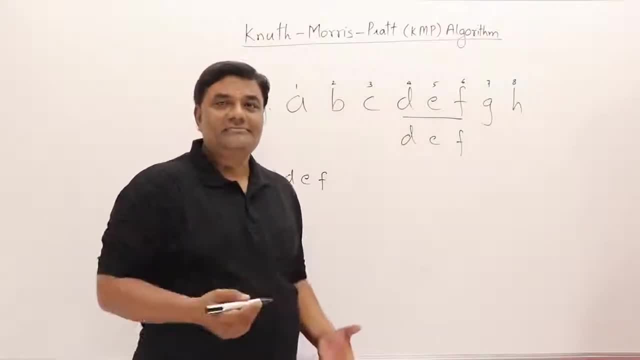 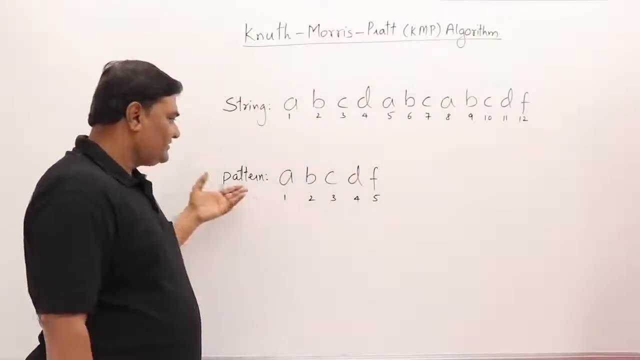 is 4 to 6 index. This example was very simple. I will take one more example and show you Now one more example Here. this is a string and the pattern that I have to search is this one. So I have to find out whether there is a match for this pattern in this string or. 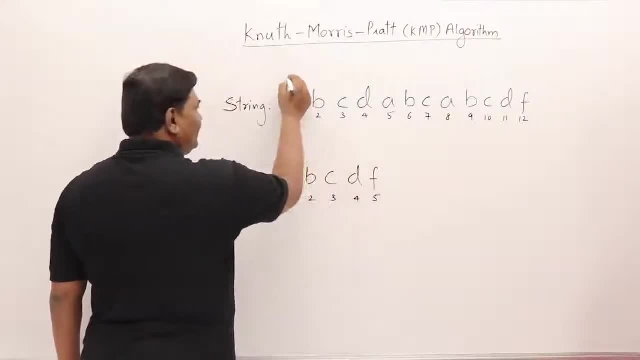 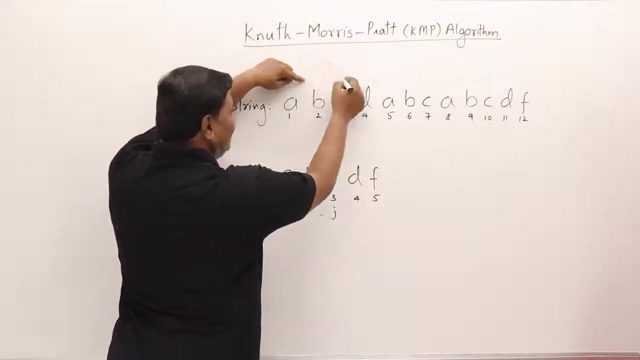 not, I will not draw a string and shift it, but instead of that I will take index i and j here. So first letter: i and j. This is matching. There is a match, So move j as well as i. So I will just write: i and j, They are matching. So move j as well as i. They are matching. 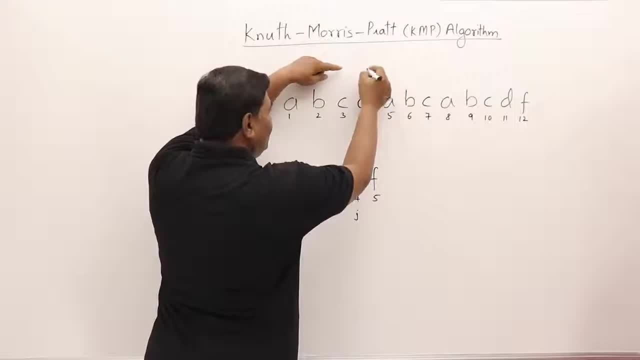 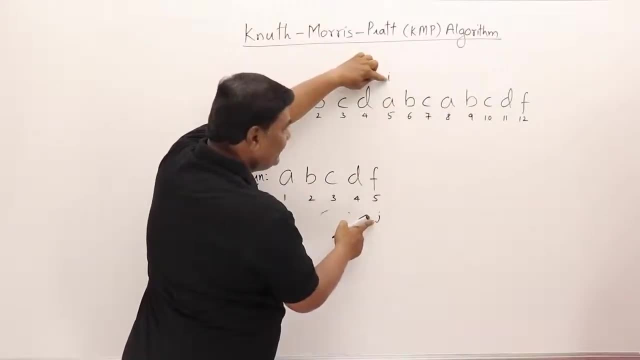 So move j as well as i. Again, they are matching. Now move j as well as i. There is a mismatch. See, we started this pattern comparing from this position onwards. As I just now said that in the previous example, I have shown you that if there is a mismatch, this pattern will move by one step. 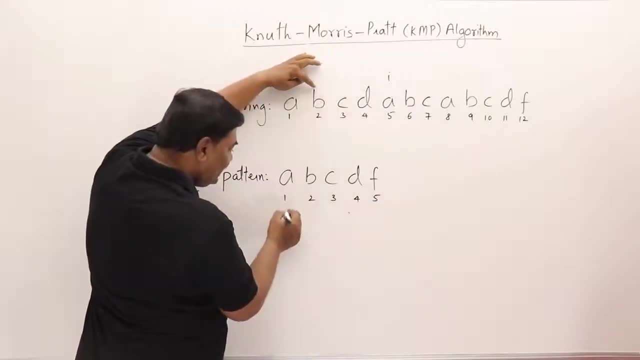 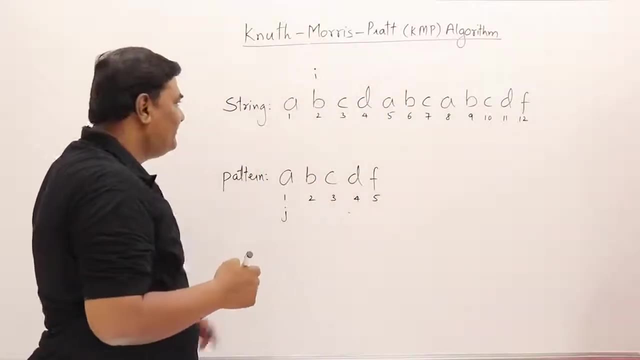 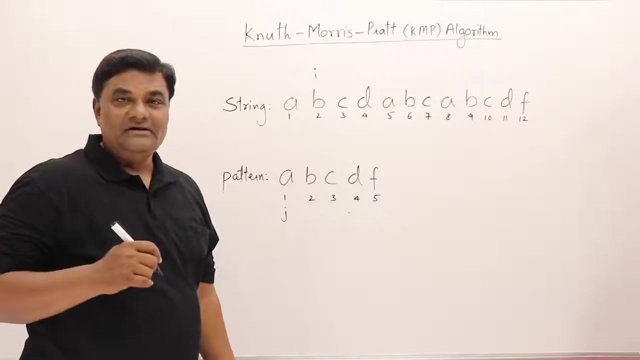 So there is a mismatch. So again, j will come in the beginning. But what about i? i will start from this place now. Already we have started from the beginning a. But what about a? Now we will start from b, That is index 2.. So this is the problem in basic algorithm. 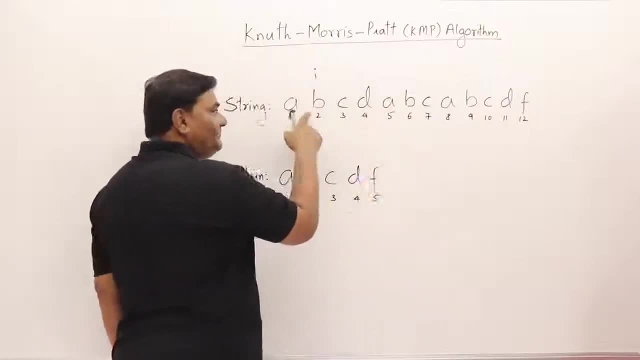 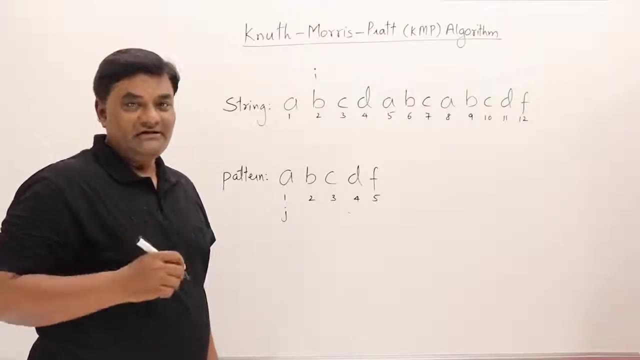 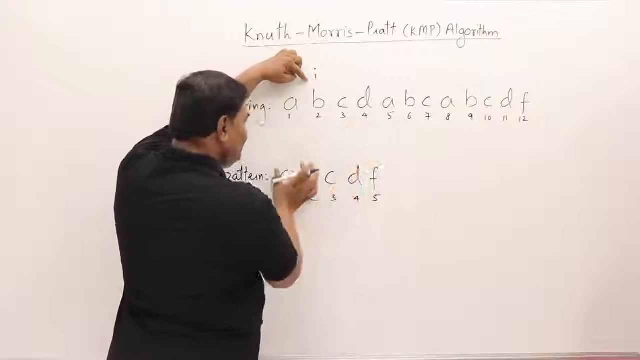 Already i have reached till 5 and it is again shifted back. So i is shifting in the string. This is the waste of time. This is the extra work in basic algorithm. Now again, we will start from here. So this means that we have started the pattern from here, now Shifted. 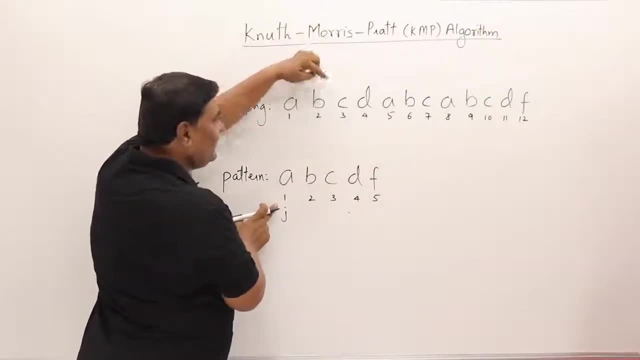 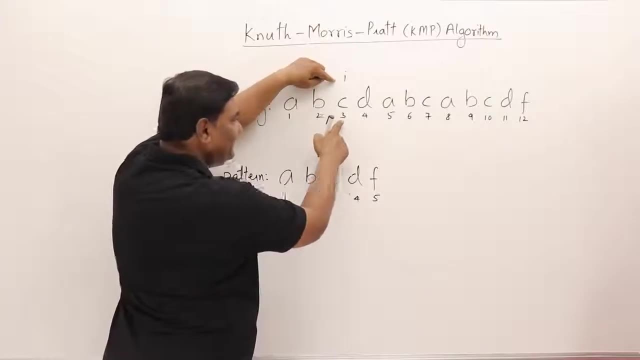 the pattern to the right by one step. That is the meaning. i came here again. There is a mismatch. So go to the next, So we will start comparing from here. So it means we have moved the pattern from here onwards now. From here we will be. 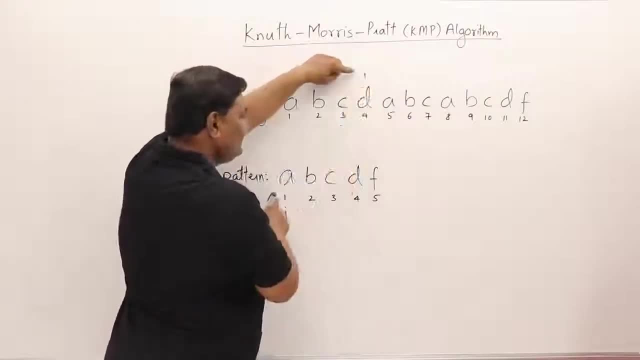 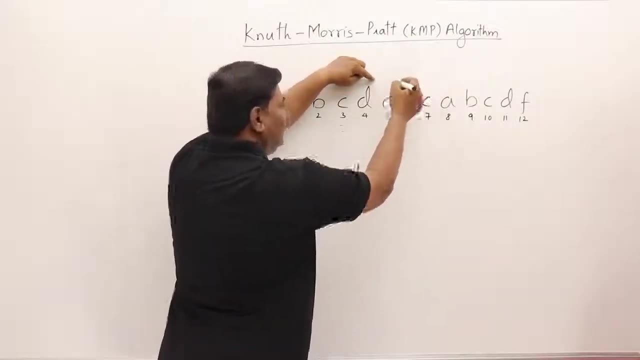 checking Mismatch. There is a mismatch, Move i. There is a match, So move j as well as i. There is a match, Move j as well as i. There is a match, So move j as well as i. 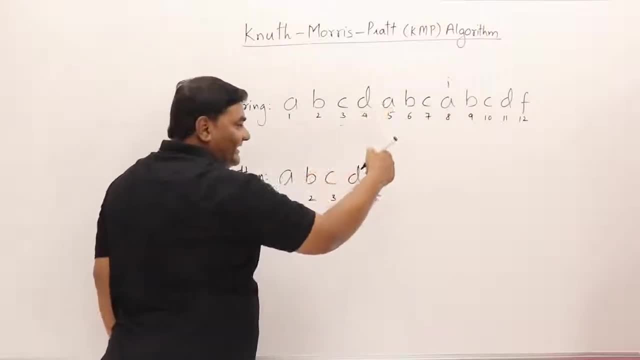 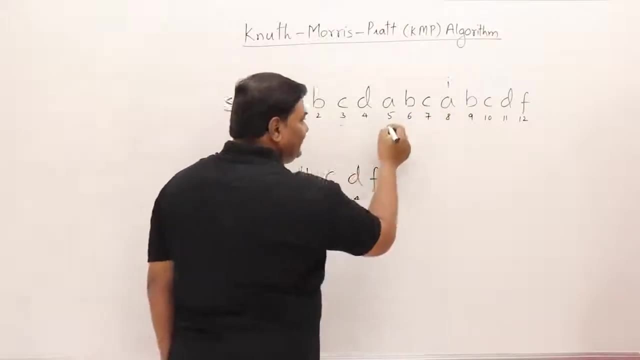 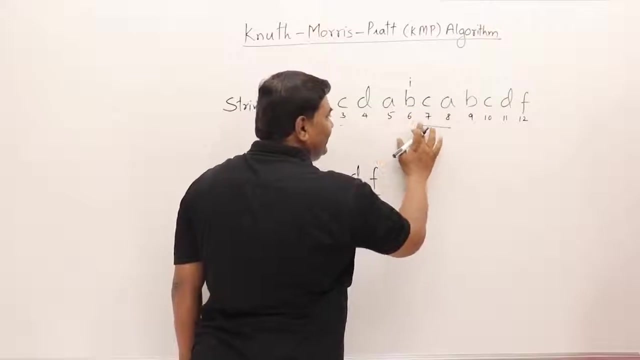 Now there is a mismatch. Mismatch means move j again in the beginning and bring i again on this part. See, just now we have started from here. Now we have to shift this one. So we will start from here, So i will come at this place. So already it has checked three. 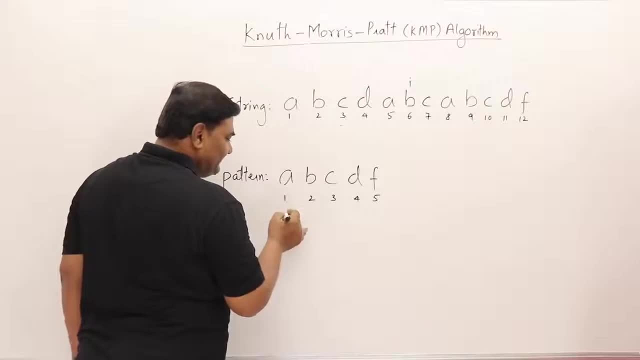 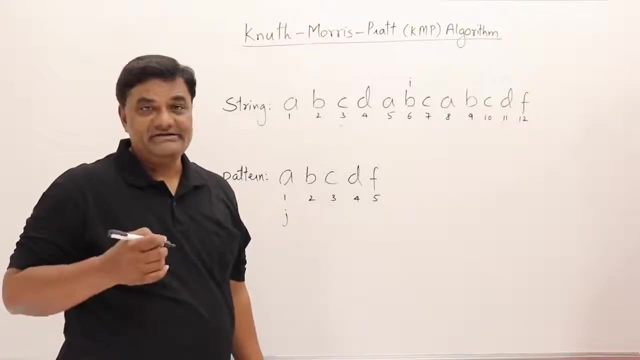 alphabets. So it should come back three alphabets. So j should start from here again. See, just now. already we have checked these alphabets. We are checking them again. So this is the drawback of basic algorithm: We are repeatedly checking the characters in the main string. Let me finish it quickly. 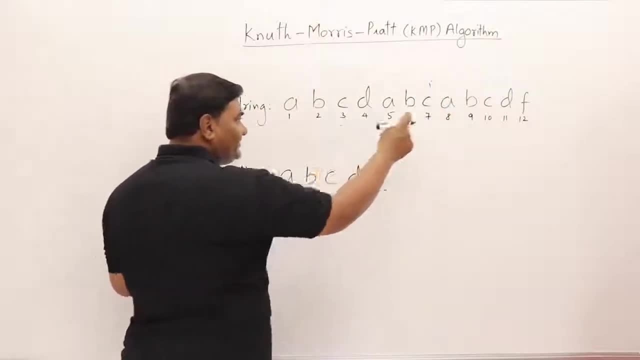 There is a mismatch, i is moved. There is a mismatch, i is moved. Now there is a match with aa. So in this way now, if I continue, then I can find this pattern here available here Every character will be matched till here. So we learn one thing here: that the 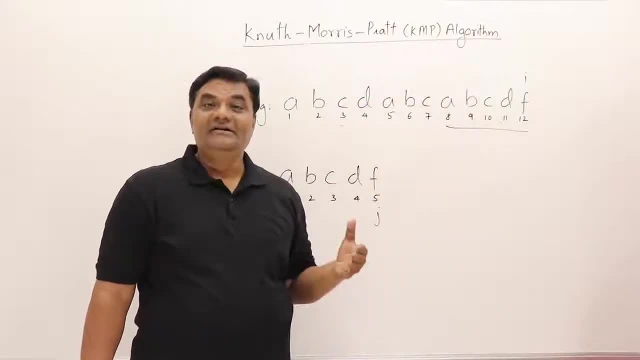 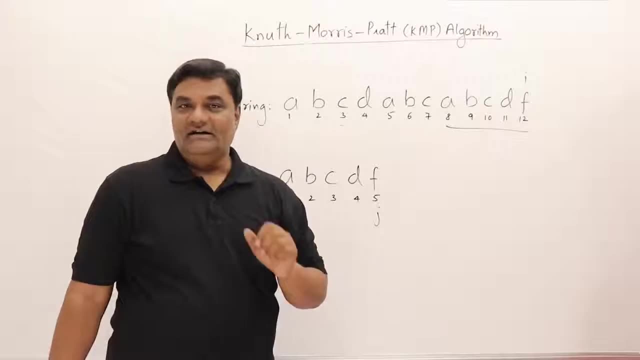 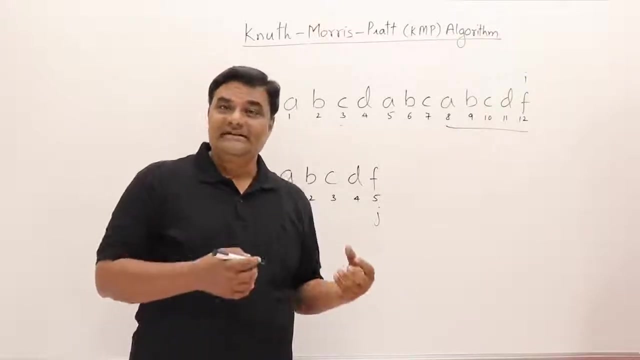 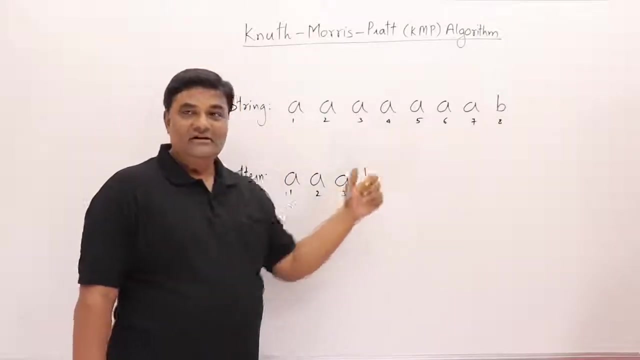 characters in the string are compared repeatedly. Whenever there is a mismatch it is shifting i, backtracking i or moving back i. So this backtracking of i we want to avoid. Let us see a worst case of basic or naive algorithm. Worst case of basic algorithm: I have a string and a pattern. Let us run basic algorithm. 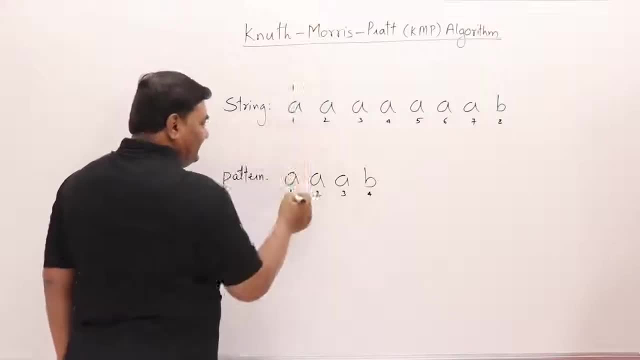 on this one: i, i, j is starting from here. There is a match. If there is a match, move i as well as. j See we started from index 1 of string. remember this: There is a match, So move i as well as. 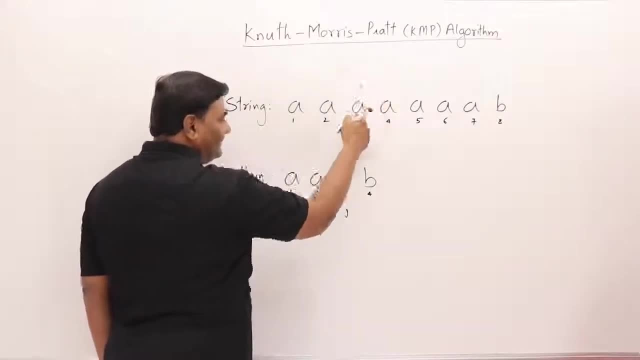 j. So first i will move j and also i will move i. There is a match, so i will move j and also i. There is a mismatch. When there is a mismatch, move j to the beginning and at the end the system is active. 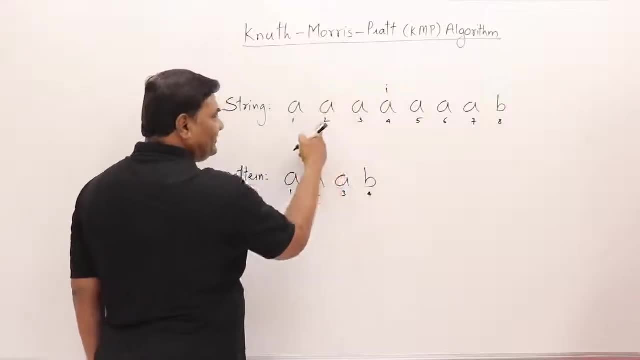 Here we have added an occurs Sh JubileeB 필. surprising step a. Move I to the second position. This is the starting point. just now We started from here, then I should start from here now. Start from here, again start. This is matching move J. 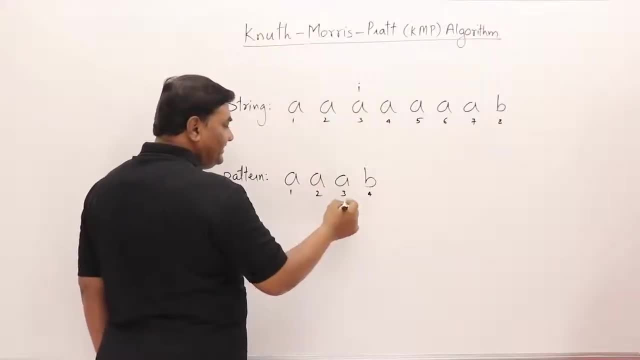 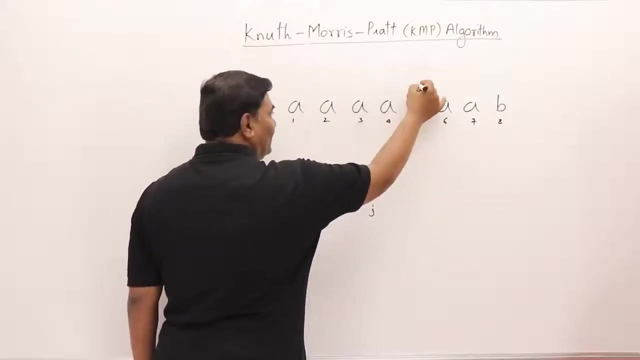 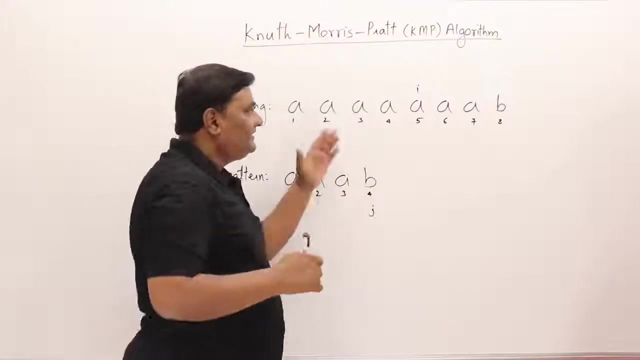 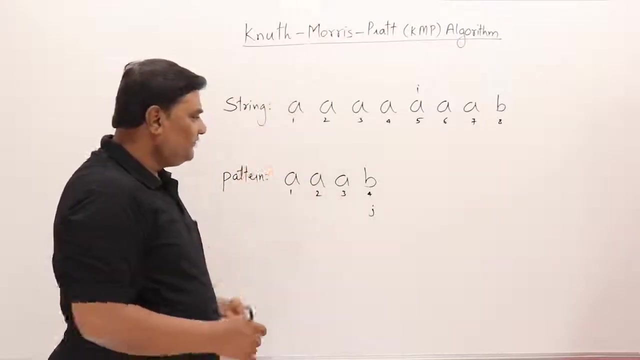 move I matching move J, Move I- again a a matching, so move J and move I. A, B is not matching, So again move J in the beginning and the move I on the third place. in this way continue. See, the problem in this one is A A. A is repeating Why I should move. 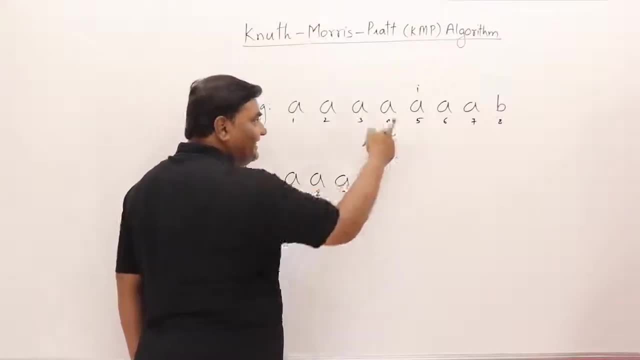 I should move just J one place and see that this is A, this is A. both are same. Just check that next alphabet is B or not. You don't have to move back and start again from the beginning, because all these are same. only That's it. That's it. 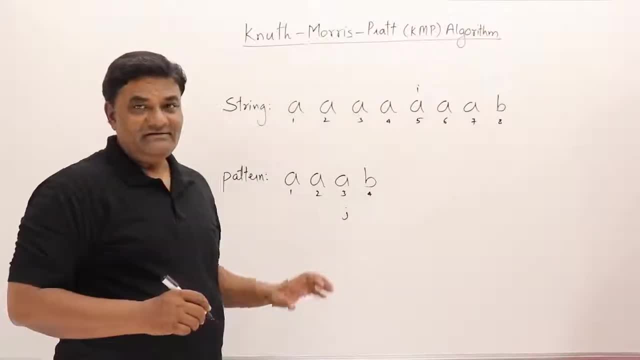 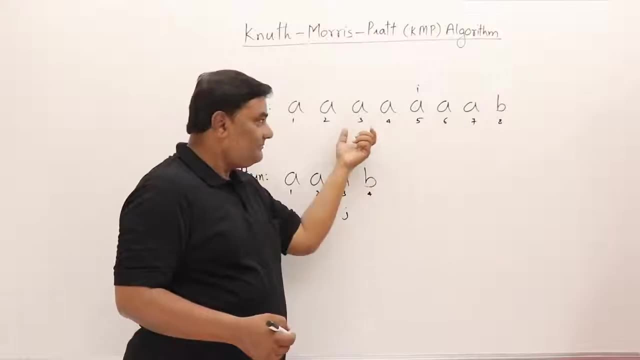 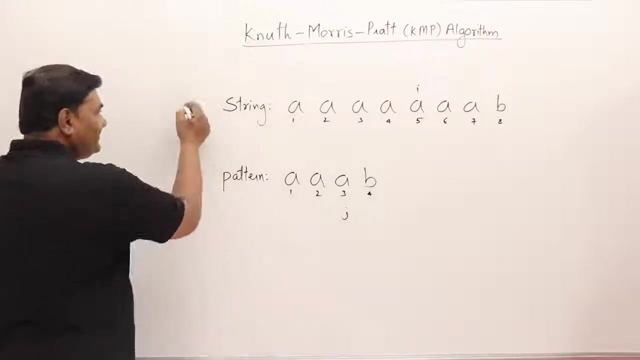 the basic algorithm doesn't study the pattern, doesn't observe what is there in the pattern, as Blindly it is checking every alphabet and just shifting this pattern by one step in case of mismatch. as this is backtracking I what is the maximum time it is taking? if the size of the string is N and the size of the pattern is? 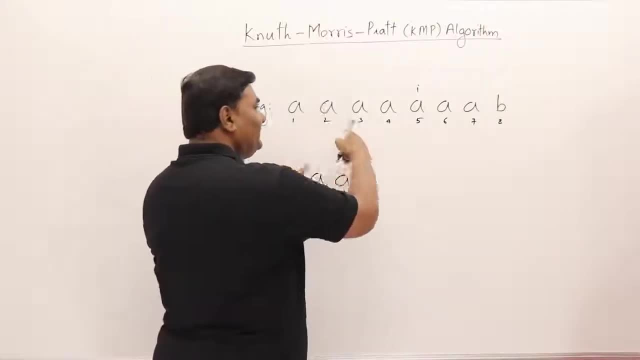 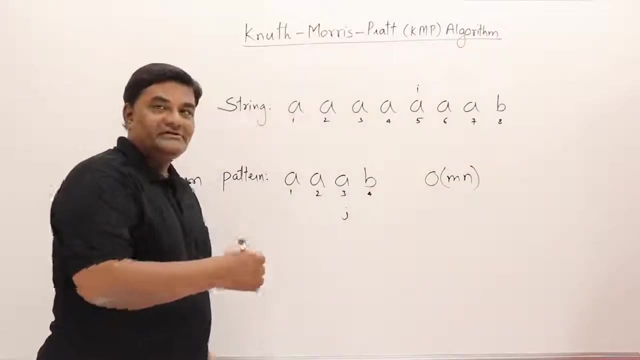 M, then almost this pattern is repeatedly compared in the string and This will be M into N. Order of M and the time. so this is the time taken by basic algorithm, A naive algorithm. basic algorithm takes order of M and time. Now can we study the pattern and reduce some time. 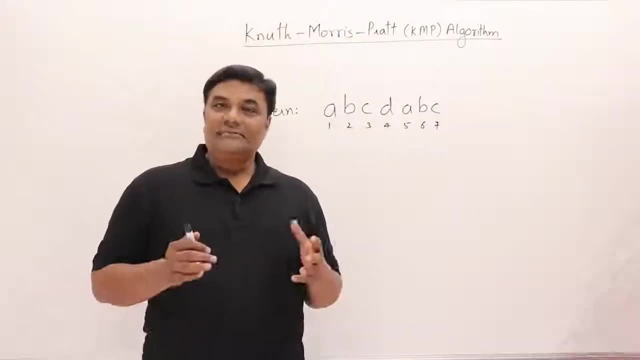 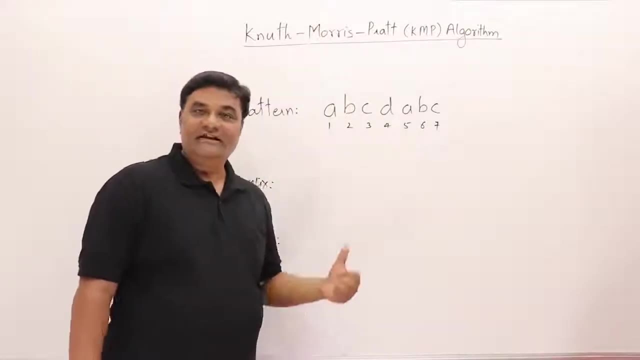 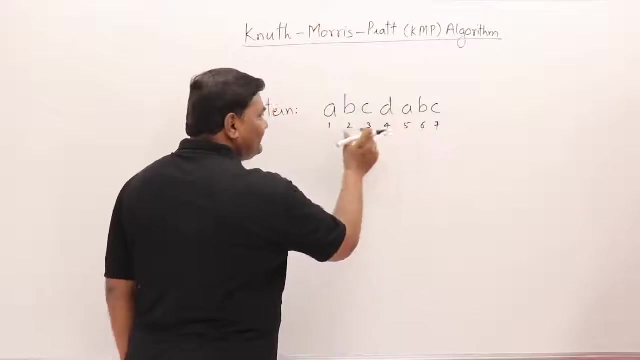 Let us see what is the idea of KMP. there is some terminology used in KMP algorithm. first Let us understand that terminology. see if there is a pattern given here, Then we will can find prefix or suffix of a pattern. So what does it mean by prefix of a pattern? we have to take the subset of this alphabets in a pattern. 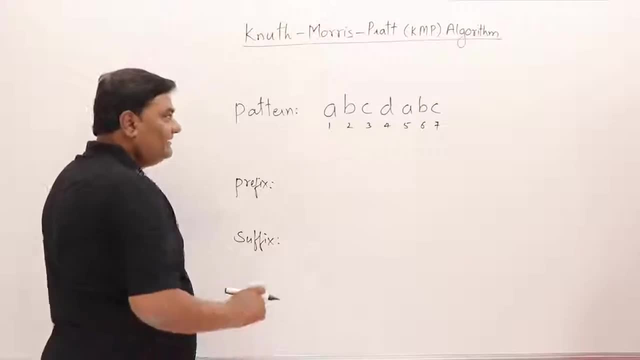 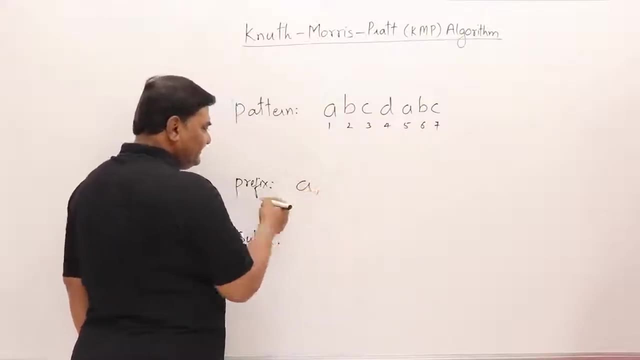 But we must start from the beginning of the pattern. only how many subset? how many characters I should take in a subset? as many as you want. So I just take a. okay, Yes, It's a prefix. No, I will take a and B Also. Yes, This is also prefix. I want to take ABC. Yes, This is also prefix. 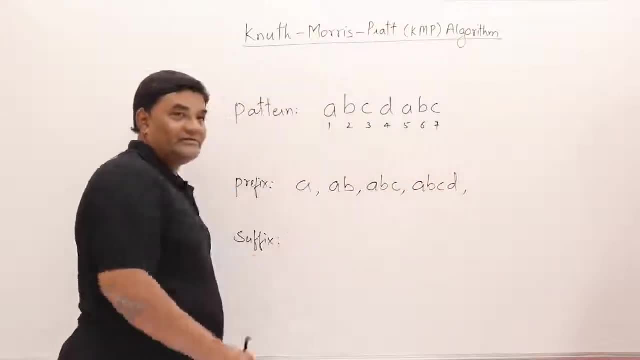 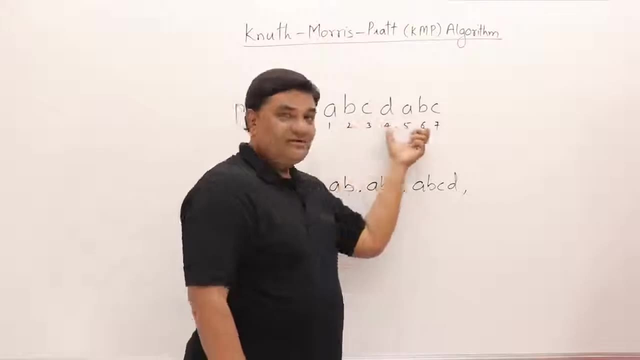 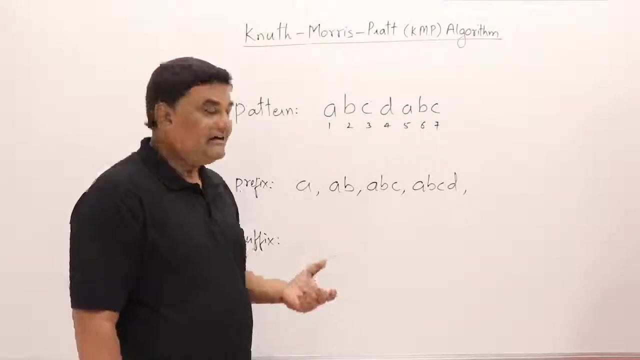 I will take ABCD. Yes, This is also a prefix. All these are valid prefix. then what about suffix? I have to take the subset of this string, but I should start from the right-hand side. only Right, and as many I want I can take. so let us start. Can I take C? just C. 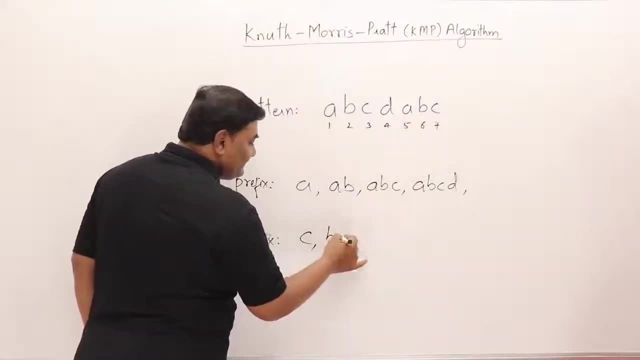 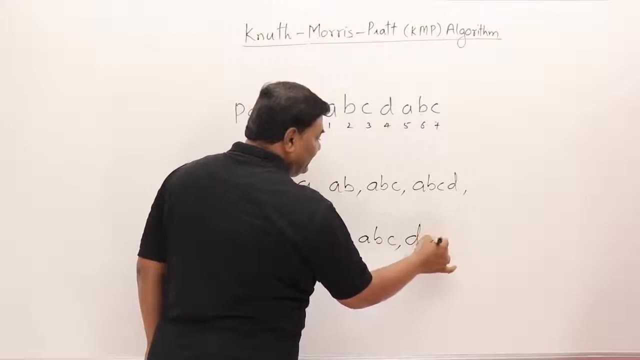 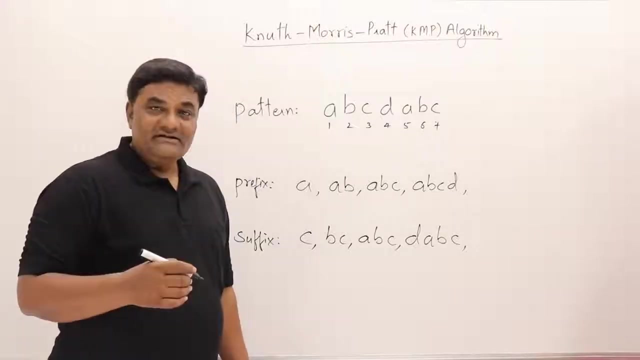 Yes, can I take B and C? Yes, BC. Can I take ABC? Yes, ABC. Can I take D, ABC? Yes, D, A, B, C and more. Let us stop here. I Now the idea of a KMP is that inside this string is there any prefix same as suffix. 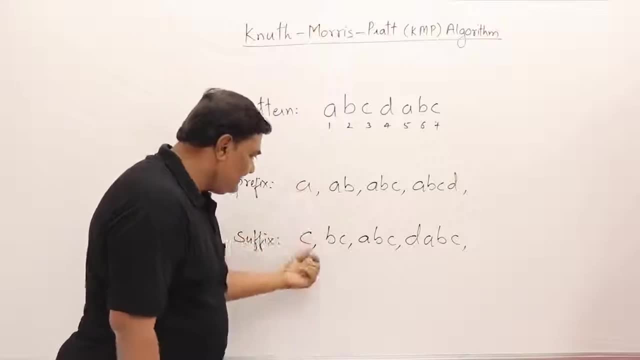 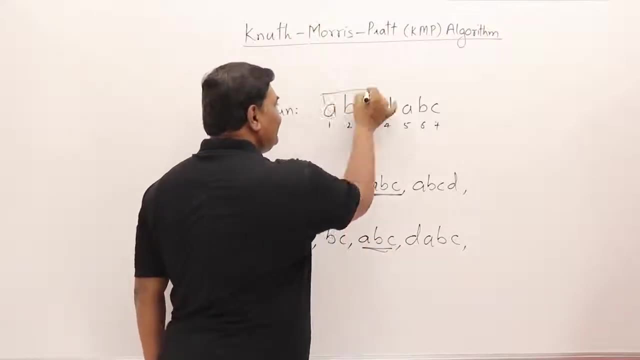 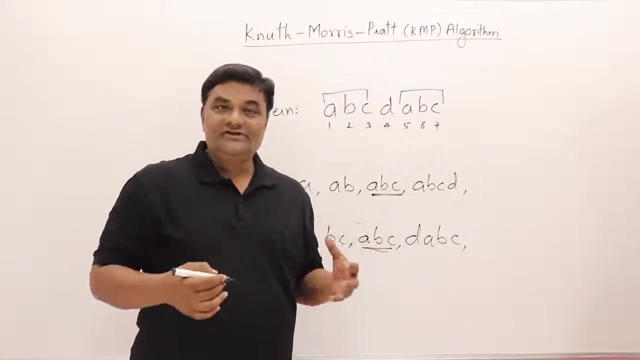 Let us see a, do you find anywhere? No, a, B, a, B, a, B. No, it's not there. ABC: Yes, It's there. See, this is matching. So this is the prefix that is also there in suffix, Also there in suffix. So this is the observation: what KMP algorithm will do on a pattern to avoid the number of? 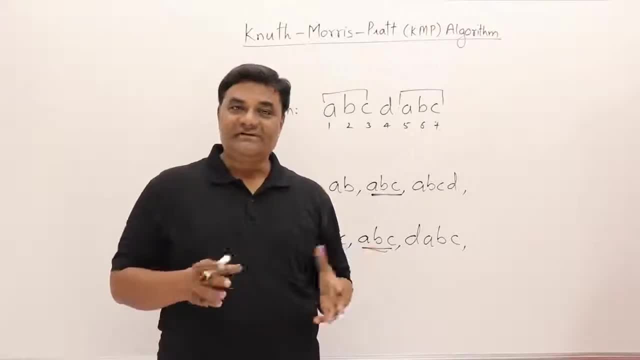 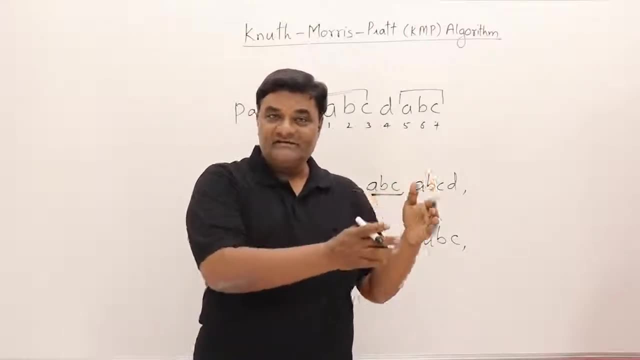 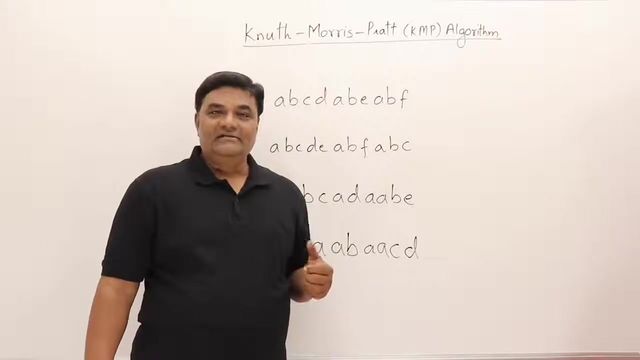 Comparisons instead of confusing with the prefix and suffix. I'll make it simple. is the beginning part of a pattern is appearing again anywhere else in the pattern or not? That's what we have to observe. I'll take few examples and show you. Let us look at the pattern and in KMP algorithm for a pattern, we generate a PI table. 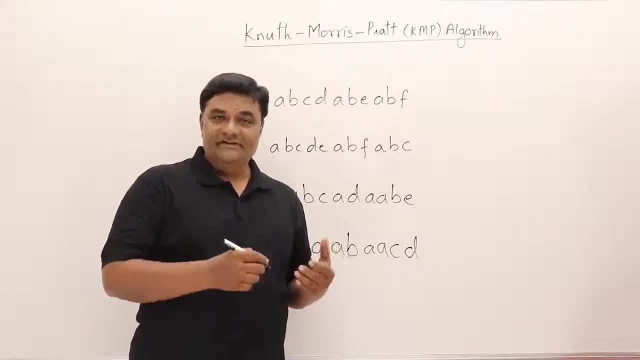 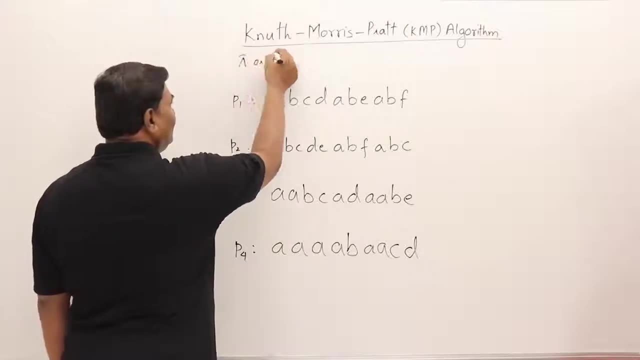 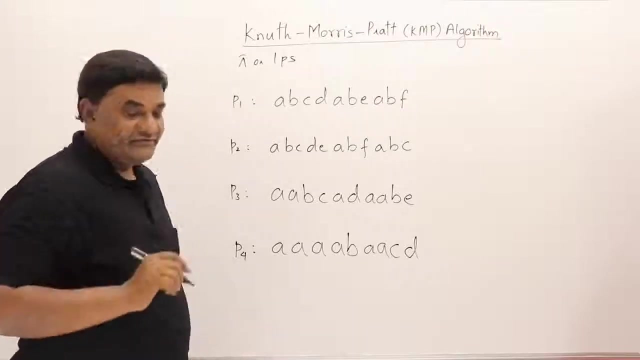 That PI is also called as longest prefix, which is same as some suffix, that is LPS. we name it as PI or LPS, whatever the name you like. So how that table is prepared, I will also show you that. just observe it carefully. Let us take first pattern. 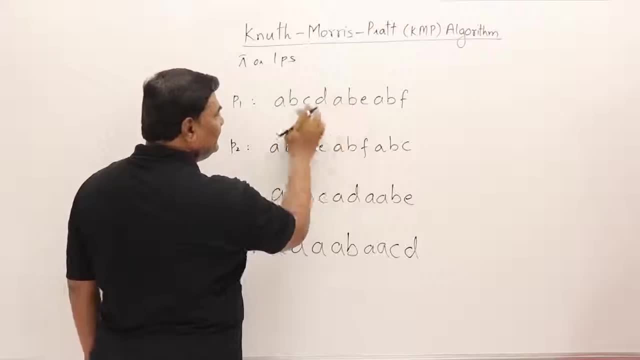 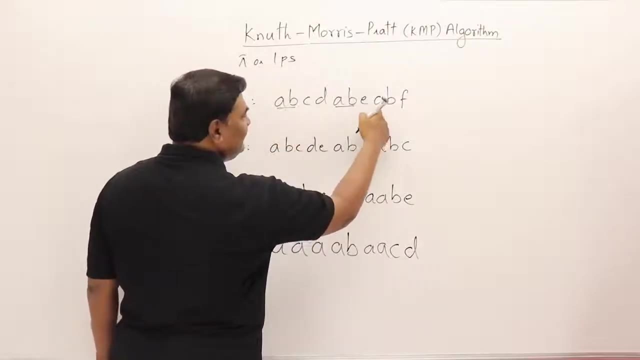 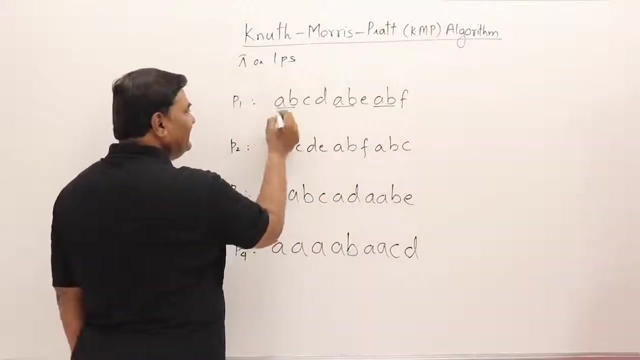 Is it appearing anywhere else? Yes, O, B is also appearing, a, B. so this a B is appearing here also. Then again a B again is appearing here. You see, a as well as B is also appearing. Okay, both are appearing again, again. So what we do is, we will prepare a table, We will write 0 0 0, 0.. This ab is matching. 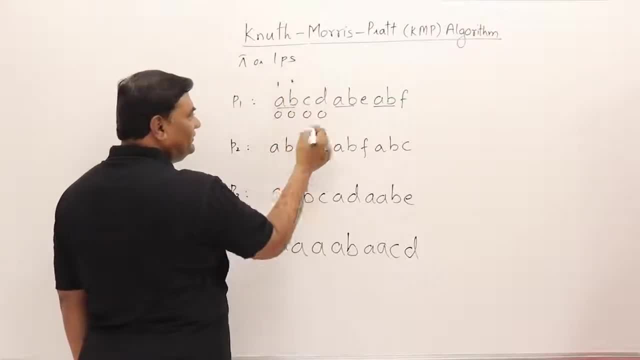 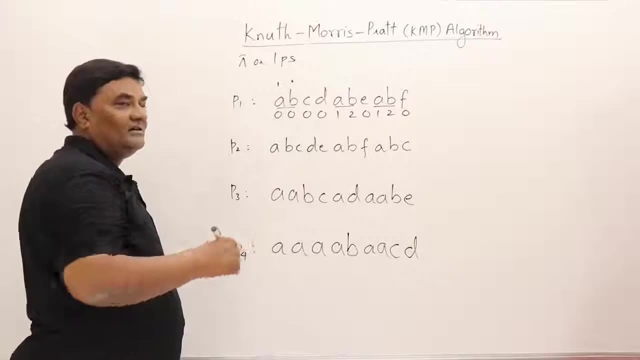 with first and second. As I said, the indices, we will start from 1 to onwards. So this is matching with 1 and 2.. This is not matching. This is matching with 1 and 2.. This is not matching. This is the pi table. Now there is an algorithm I don't want to show you. 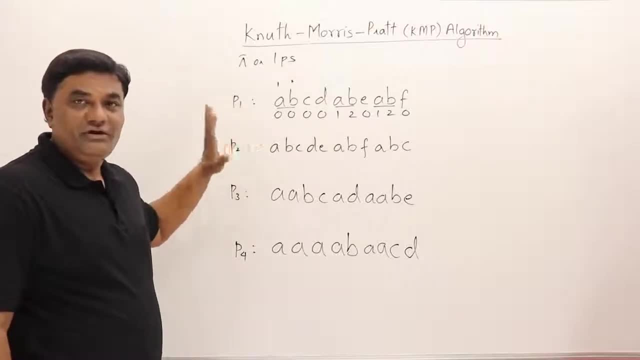 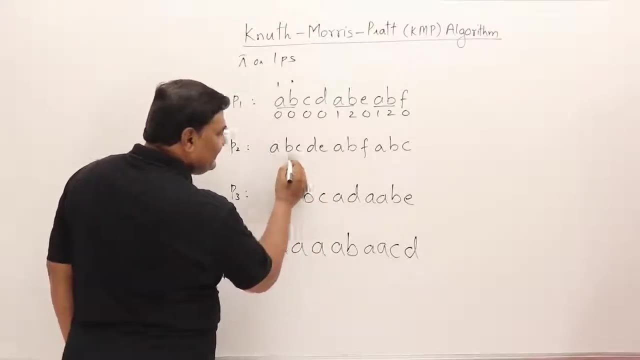 that algorithm. I am not tracing the algorithm, Simply I am showing you how to prepare it. If you trace the algorithm, you will get the same results. Next, let us look at this pattern. A- is it appearing anywhere? Yes, it's appearing. O, b is also appearing, So this is matching. 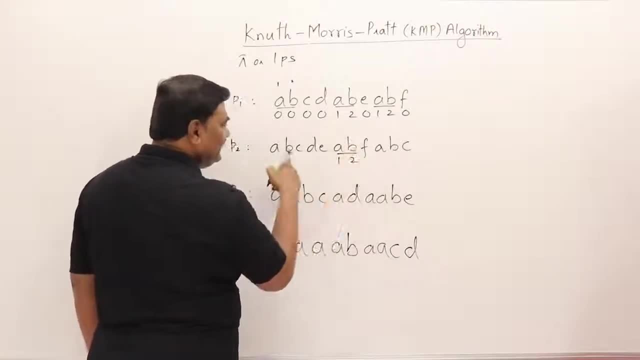 So this is 1 and 2. Then a anywhere- yes, it is appearing here. So b, c is also appearing. So these three are matching 1, 2, 3. Rest of them are all zeroes. That's the pi table. 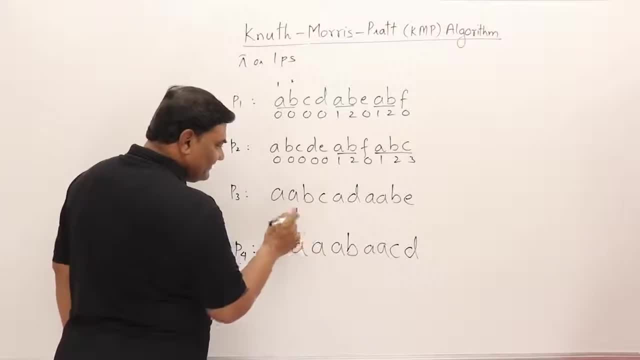 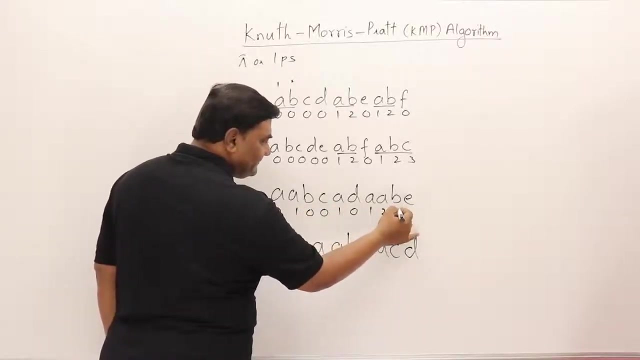 Now let us check A. is it appearing anywhere? here itself? So mark 1.. A is it appearing? Yes, it's appearing. then next alphabet: no, it's not. same a is appearing here. the next alphabet also matching 2, then rest. all of them are zeros. what about this? a is appearing. 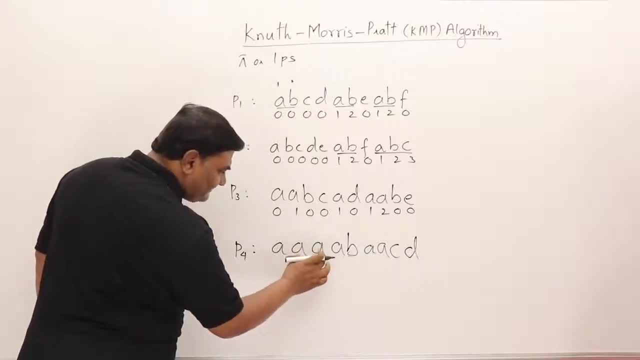 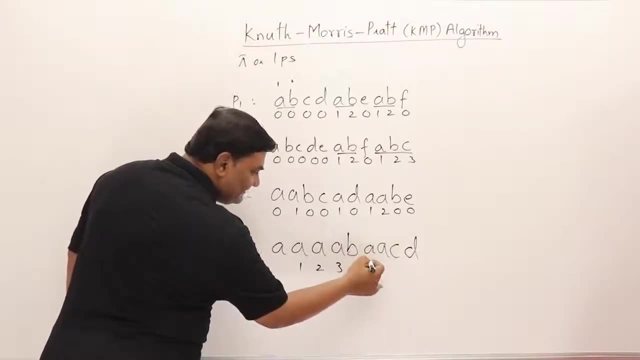 here 1 and this a is also appearing, so from here, if you take, this is matching with this 2, so 2 and these 3 are matching with this 3, so take 3, then anywhere else. yes, a is appearing here. the next a is also same, so 2 and rest. 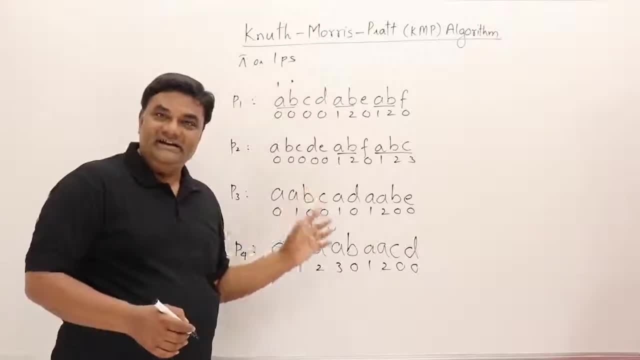 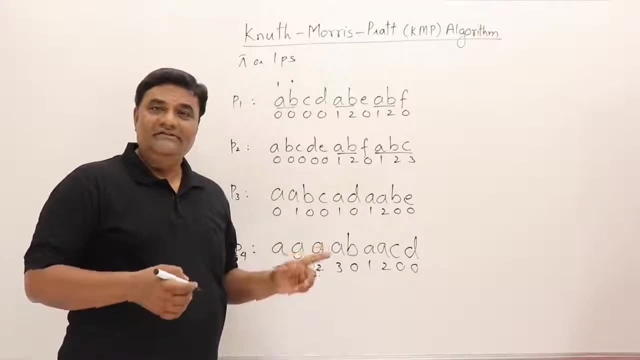 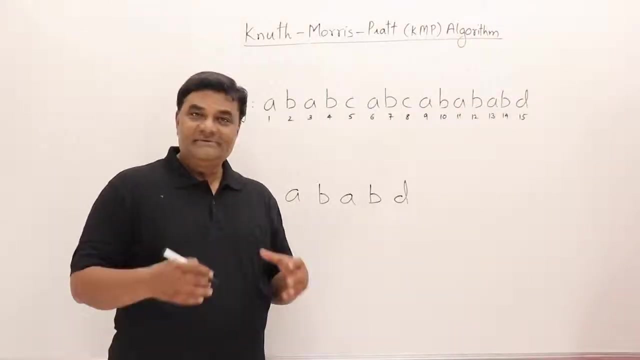 of all the values are zeros. so this is the base of KMP algorithm to prepare the table. once you prepare the table, the algorithm is simple. then I will take one example and show you how algorithm works. let us look at the working of KMP algorithm. my explanation will be based on the tracing of an algorithm, so one. 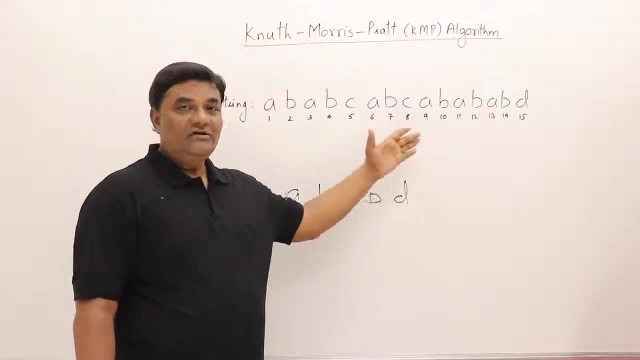 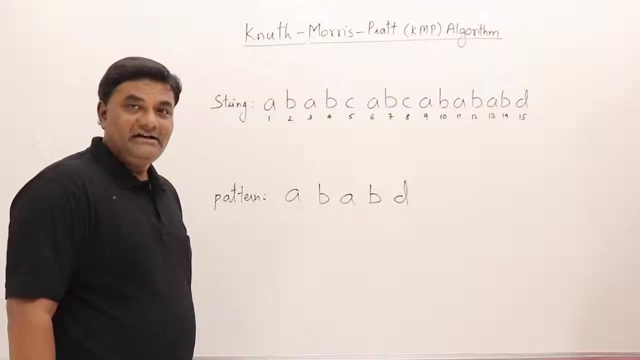 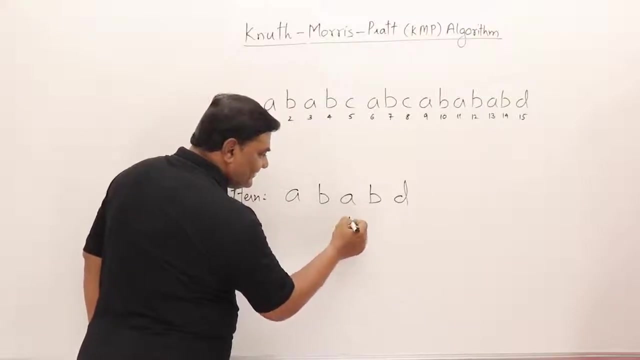 thing you have to observe that here in the string we will not backtrack in the main string, so let us start the working. so this is a pattern. so first of all prepare a PI table or LPS, so prefix table a. this is appearing here, so this is one. the B is also there. 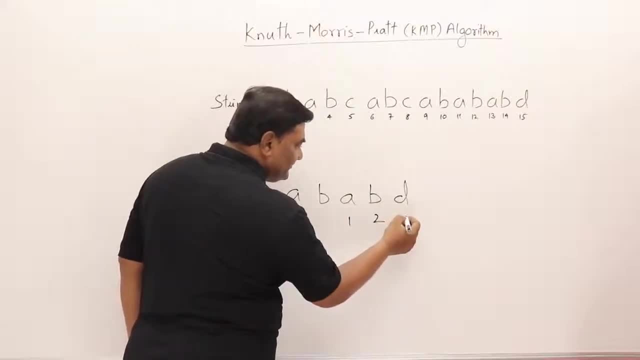 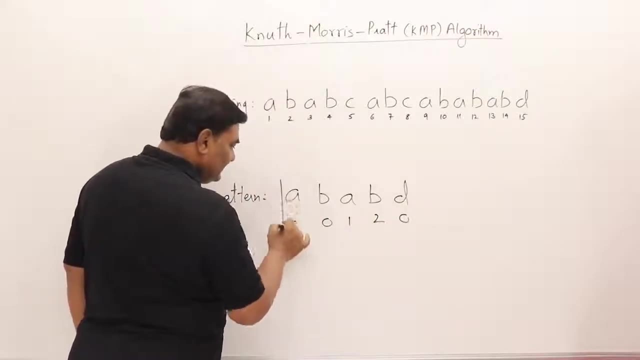 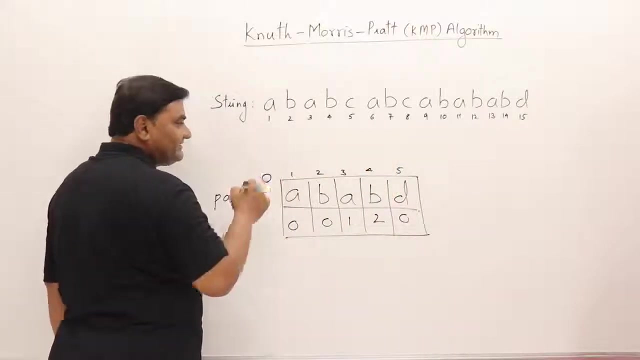 so 2, then D is not matching here, so not just just two alphabets are matching. so take this as 0. this and this all are zeros. so let me put it in a table like this: so give indices 1, 2, 3, 4, 5, and also I will take one index, 0, that will act as a. 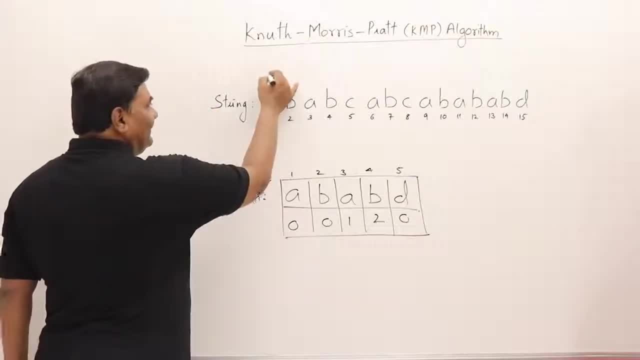 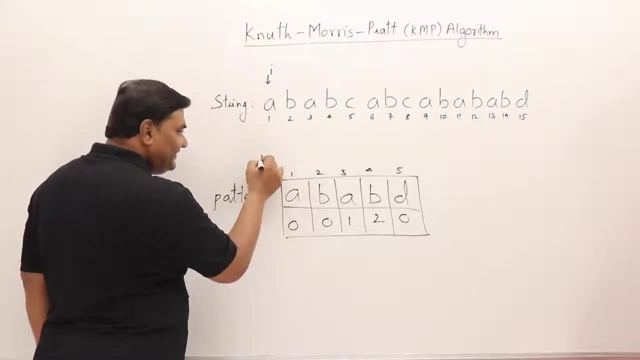 starting point of a pattern. now let us start first alphabet. I is there, then where is J? now it is, it is not on the first alphabet. we will take it on 0. this is a special thing. you can start from here also, but the working will change a. 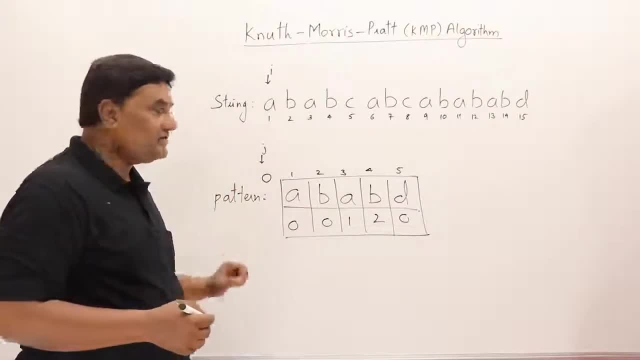 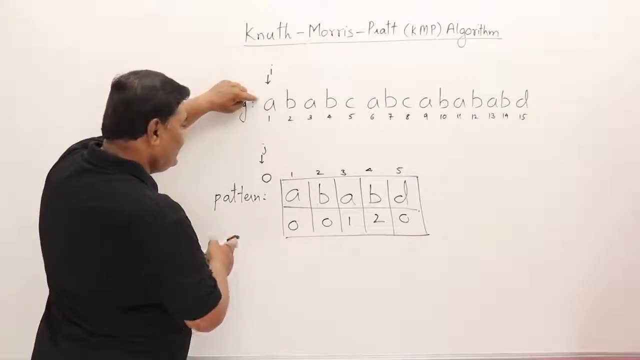 little bit. I am starting from 0. this is easy. let us watch. how is this? J is on 0, eyes on one. first alphabet. now compare this string of I with the pattern of J, plus one being here. check the next alphabet. they are matching. if they match, then the move J as well as I. now again compare string of. 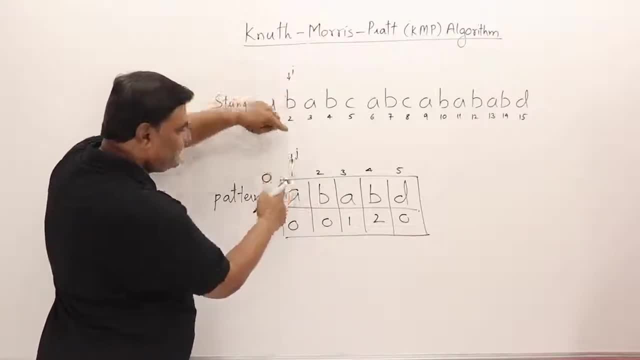 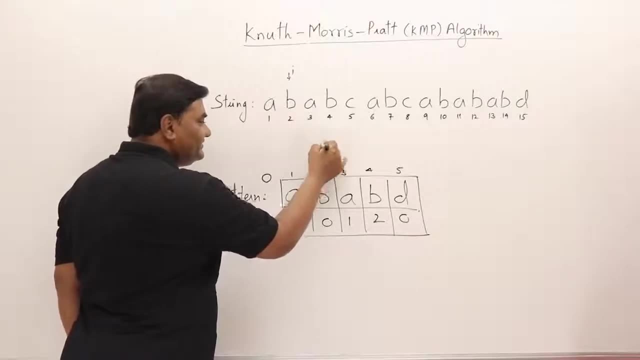 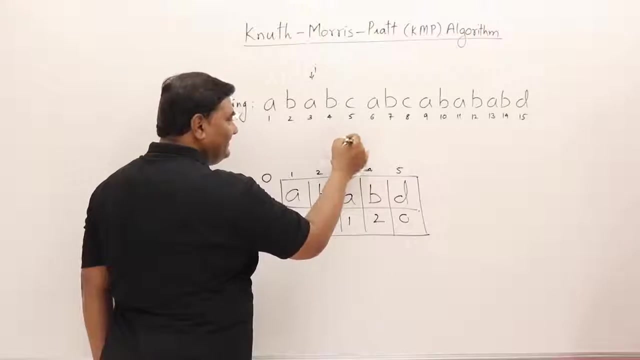 I with the pattern of J plus one, this alphabet. so wherever Jay is pointing, you try to check the next alphabet. thus BJB's here. so take J on the next and I also on the next. now this J plus 1. yes, this is matching. this is matching J plus 1. so move J as well as I. now J plus 1 is B. 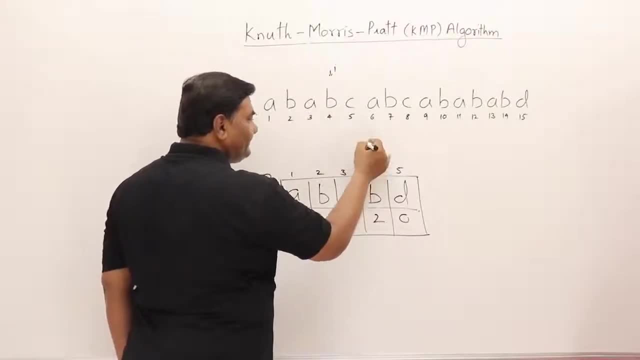 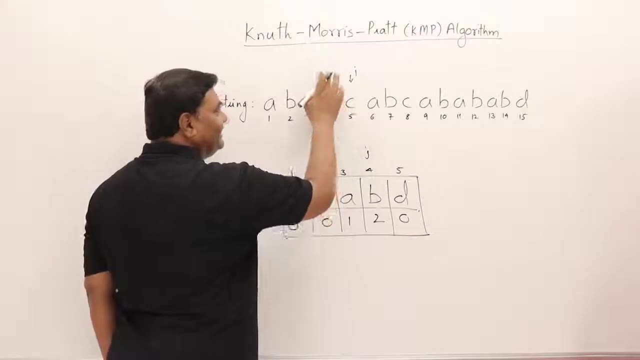 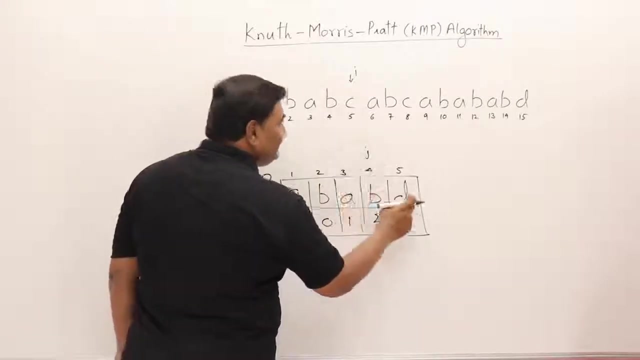 and I is B. they are matching, so move J as well as I. now J plus 1 is not matching with I, so now there is a mismatch. what to do? observe it carefully when there is a mismatch with J plus 1 and I then move J to this index to bring. 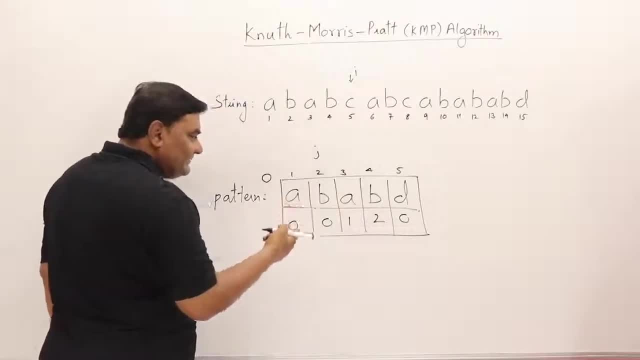 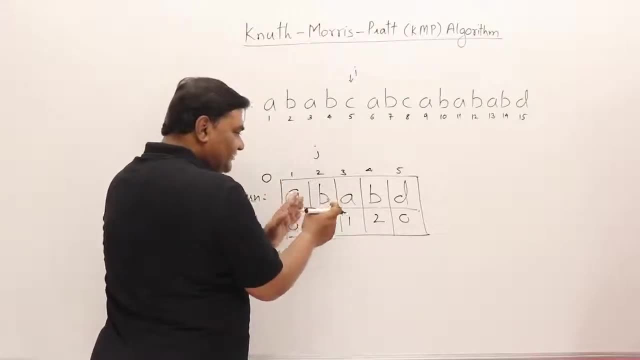 J here here. move it here. this means that this AB, AB is repeated, tripling as Okay. So AB came two times. So already we have checked one time, So maybe we have to start from here. So let us observe Now: J plus 1 with this one, Is it matching? No, still there is a mismatch. So again, move J to this place. 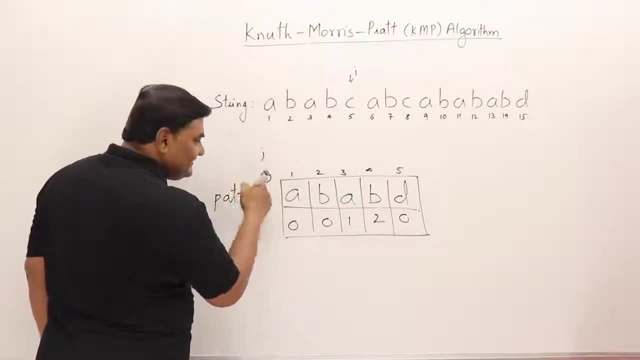 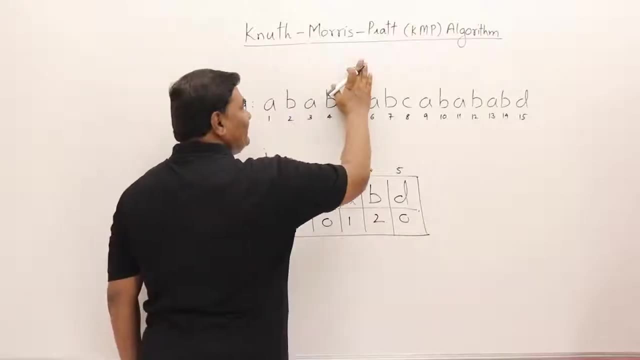 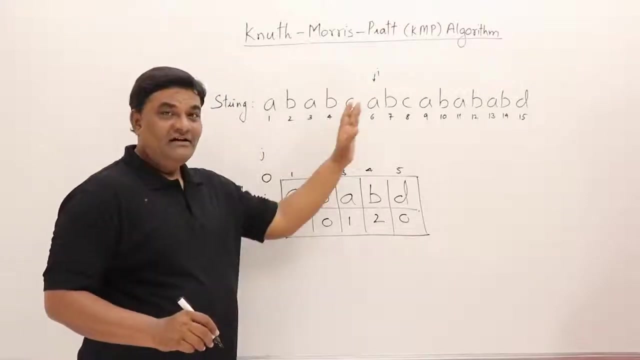 J is here Now is it a match with J plus 1?? No, still there is a mismatch. but J is on 0, So we cannot move J further, So move I. So in case of mismatch, you observe that only J is moving. I is not backtracking. 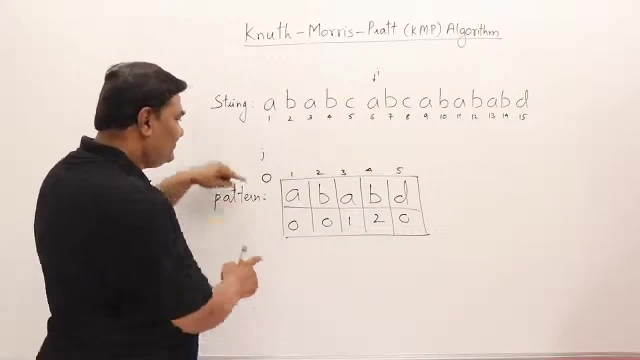 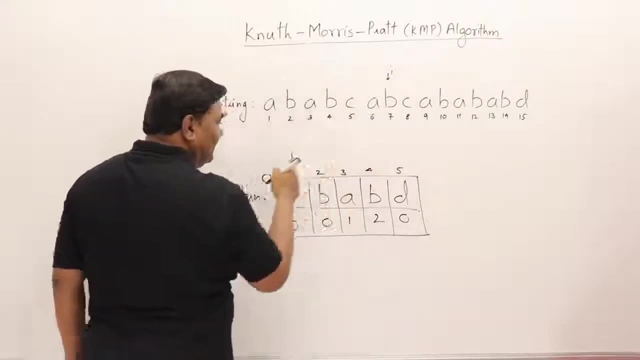 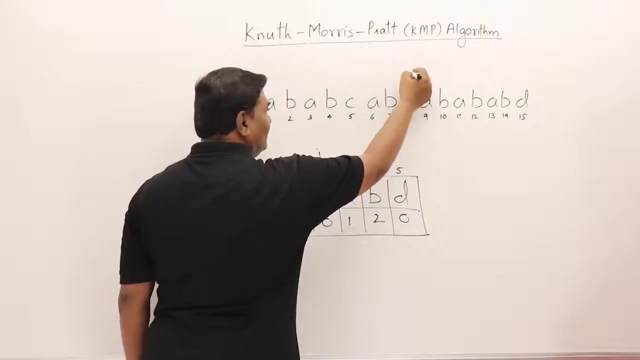 I has simply moved to the next alphabet. Let us continue. J plus 1 is a match with this. I so move J, move I J plus 1. B and I is B match, So move J and move I. J plus 1 and I C. 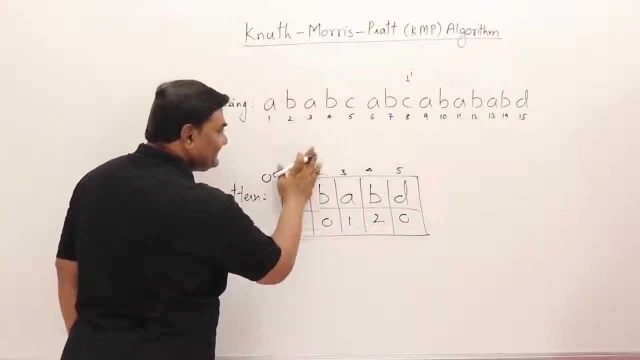 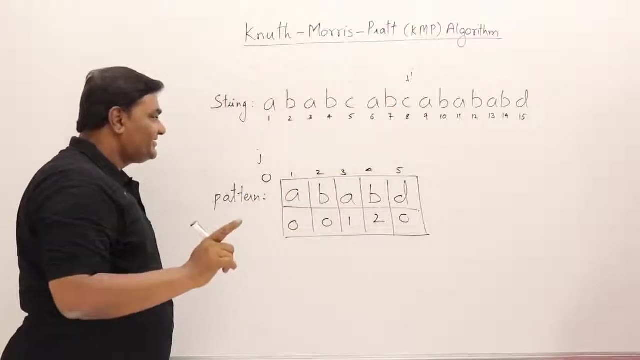 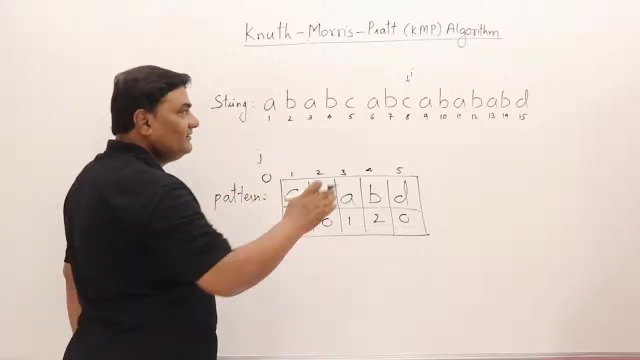 A mismatch. so move J to this place, J, and still compare J plus 1, A and I Mismatch. now there is a mismatch and even J is at 0, so we cannot move J further on the left, So just move I Now here this part you observe carefully. 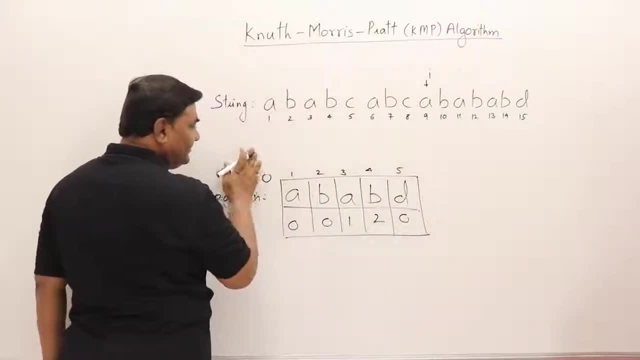 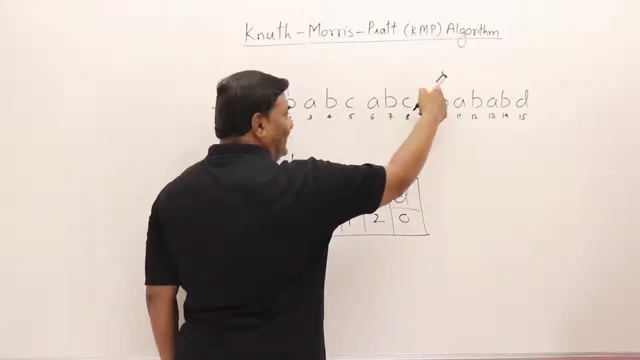 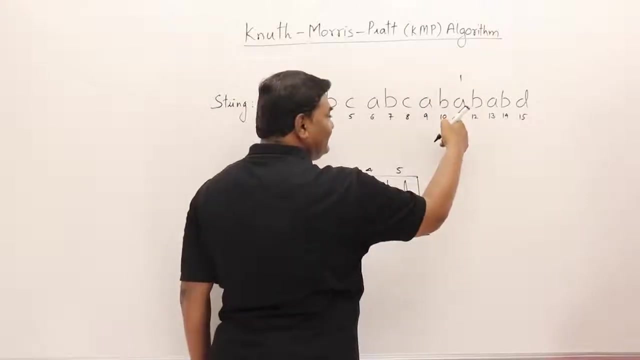 J plus 1: A- I. this is matching. move J, move I. This I'll mark here now: J plus 1 is B and I. they are matching, so move J and move I. J plus 1 is a and I is a matching, so move J and move I. 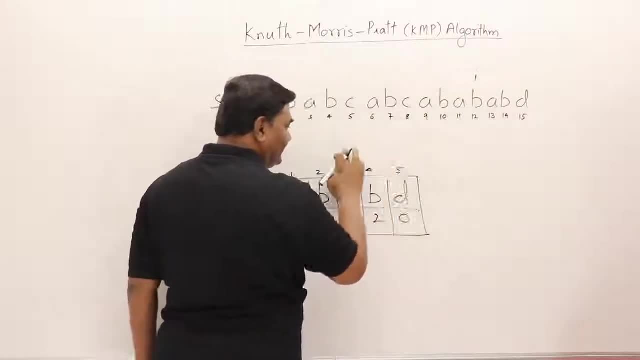 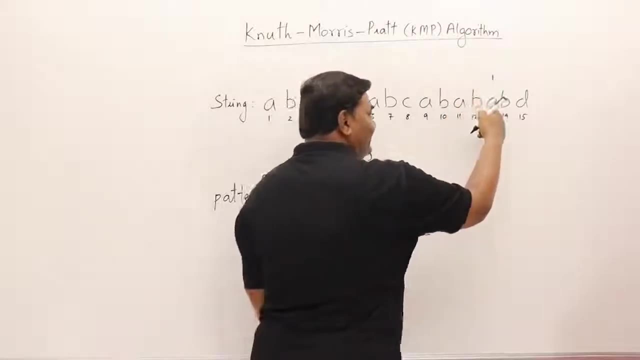 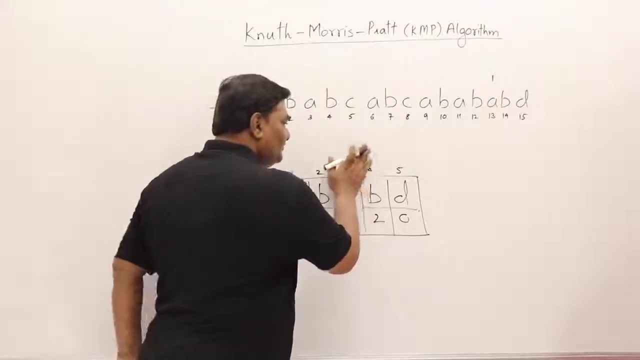 J plus 1, that is B and I. they are matching. so move J and move I. J plus 1 is a, D, but this is a. they are not matching. They are not matching then where to move J? at 2, 2. Then again compare J plus 1, a: a. 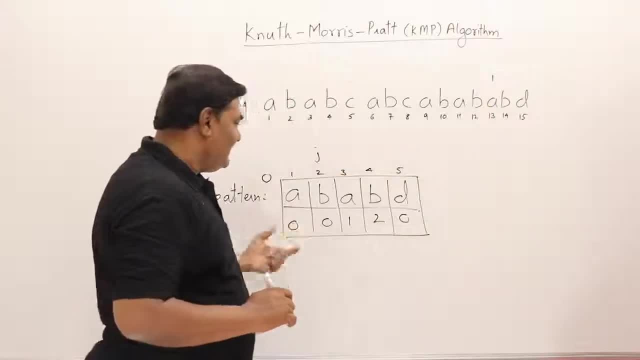 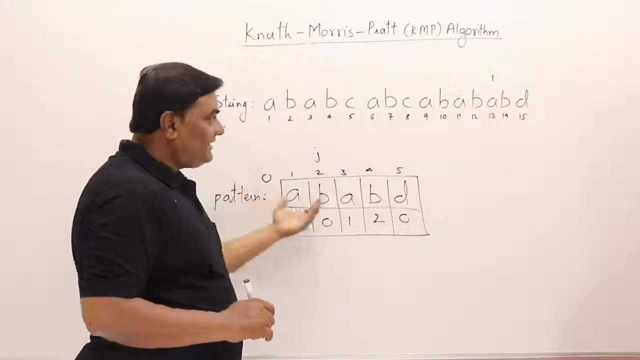 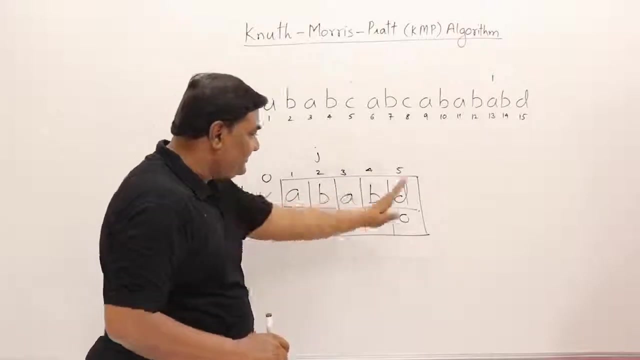 match match C: a, B, a B. So a B already. this portion is a B and this is also there here, So we need not compare that. we can continue from this portion here. This was a mismatch. You can again start from the beginning. means we reach till here. means this: a we have.